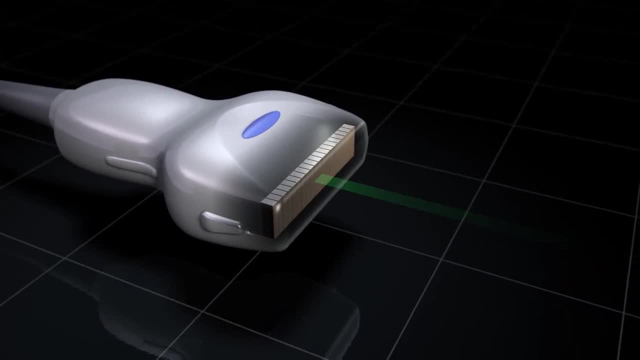 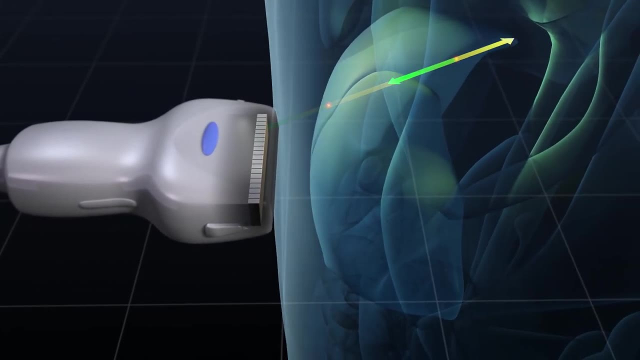 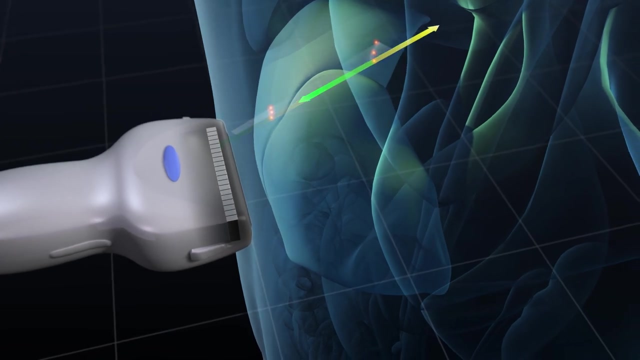 This is a device that generates and transmits ultrasound and also receives the reflected signals. Every time this ultrasound enters or leaves organs and tissues inside the body, some of it is reflected back as an echo. By picking up and analyzing these echoes, a diagnostic ultrasound system can build up. 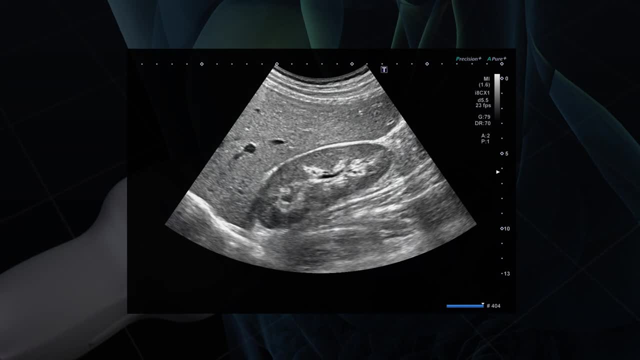 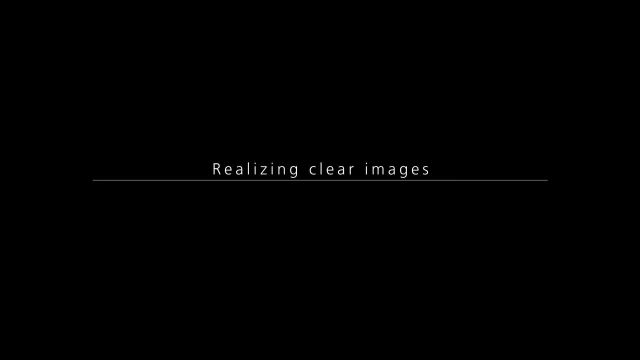 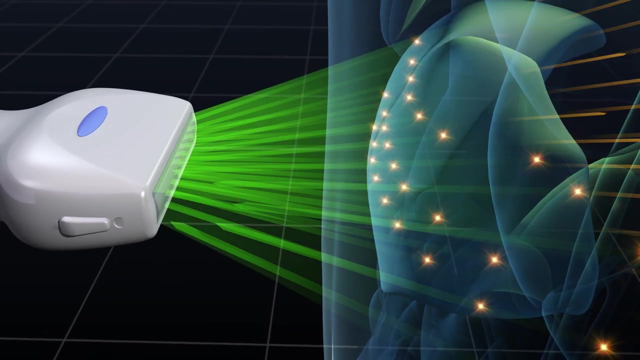 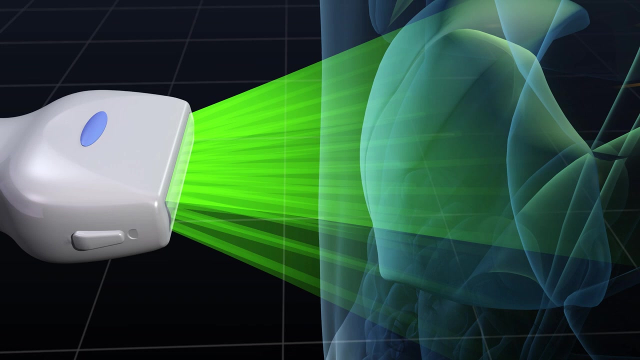 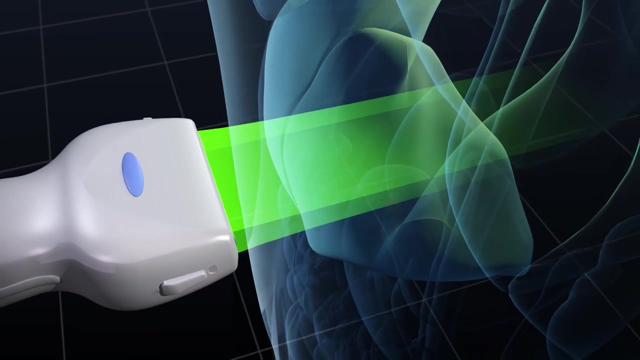 an image of these organs and tissues. Ultrasound emitted from the probe can be reflected from many places, so the reflected signals also contain a lot of unnecessary information. Steps are generally taken to reduce this unnecessary information by receiving a narrower, sharper beam of ultrasound signals. 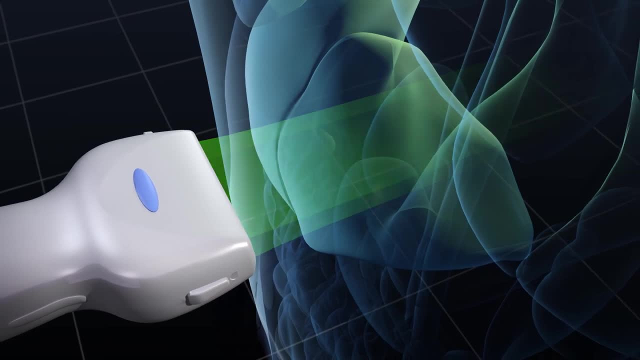 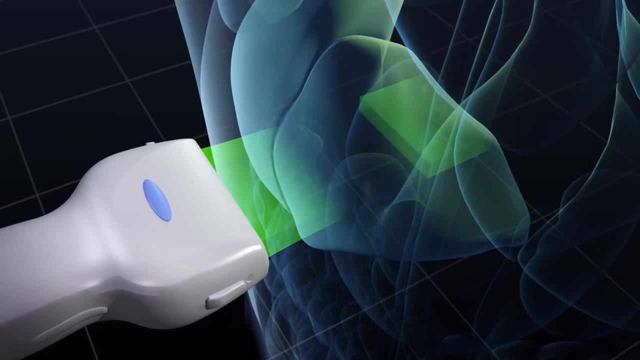 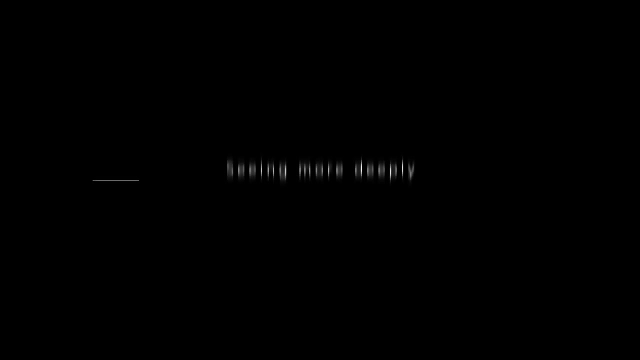 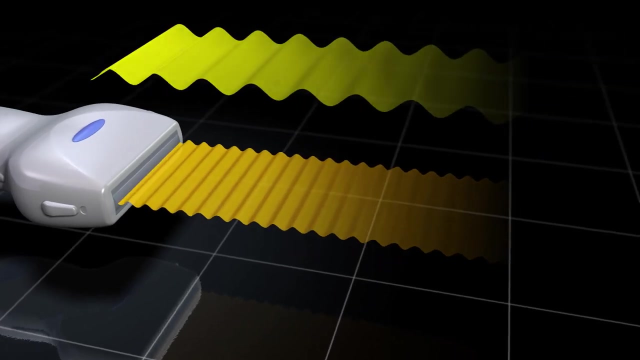 This results in images with greater clarity and detail. However, the further ultrasound travels, the weaker the reflected signals are. This can make it difficult to obtain clear images of deeper parts of the body. Canon has developed a technique in which two different ultrasound frequencies are combined. 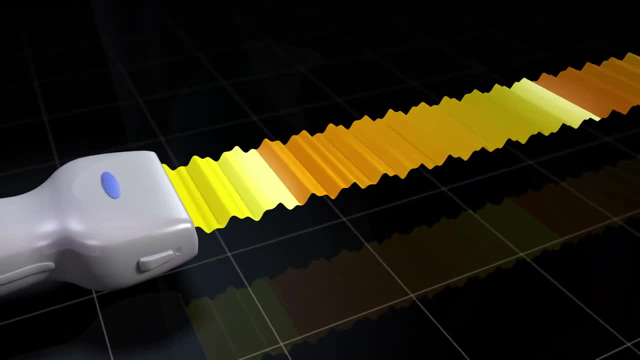 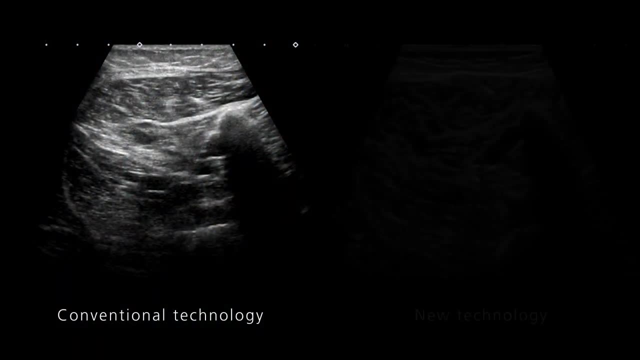 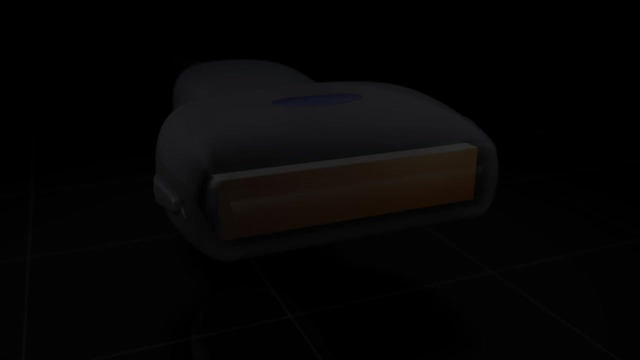 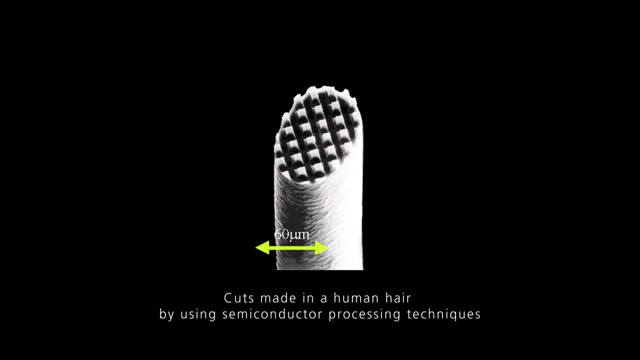 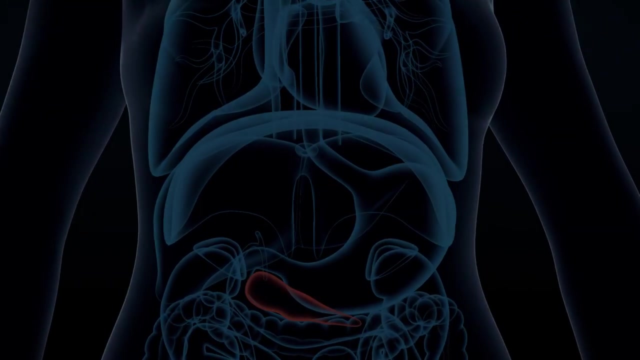 and transmitted simultaneously, This new form of ultrasound signal can penetrate further into the body, resulting in images with excellent detail. By using semiconductor processing techniques to produce the sensor parts of the ultrasound probe, we are able to obtain images with greater definition. These technologies have made it possible to use ultrasound diagnosis in a much broader 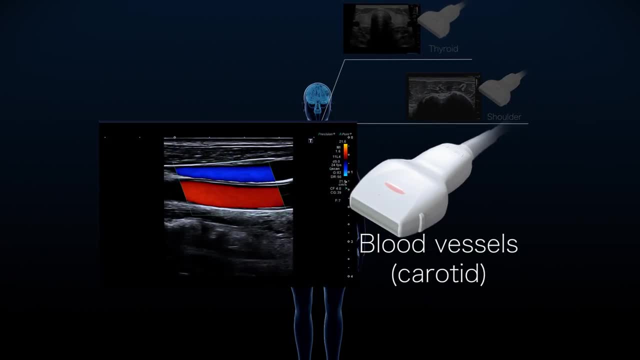 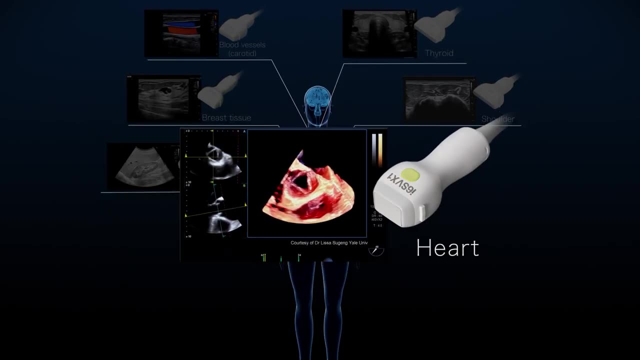 range of patients. We have also developed a wide range of technologies that can be used in the field of ultrasound diagnosis. We have also developed a wide range of probes for different parts of the body. Since ultrasound is non-invasive and involves no radiation exposure, it is suitable not 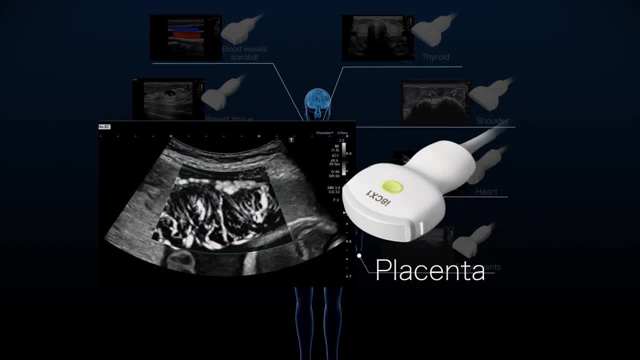 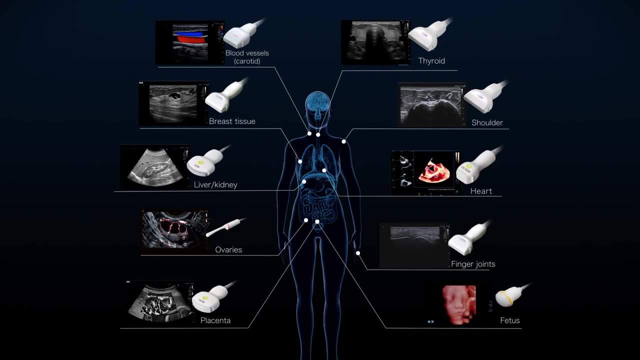 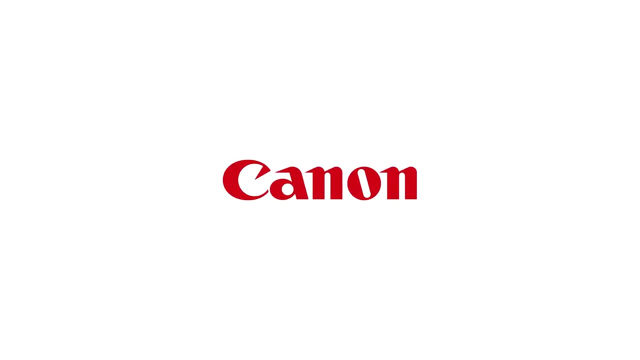 only for the early detection of tumors and lifestyle-related diseases, but also for a wide range of medical fields, including gastroenterology and orthopedic surgery. We have developed a wide range of technologies that can be used in the field of ultrasound diagnosis.